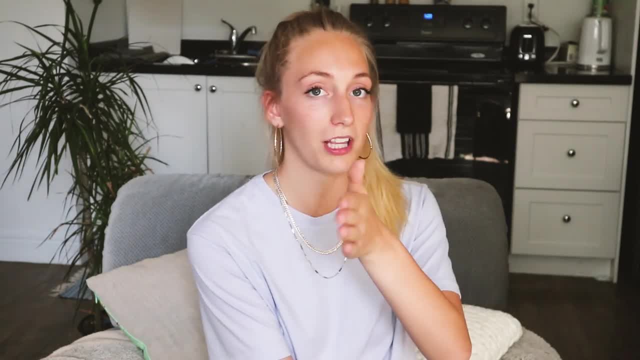 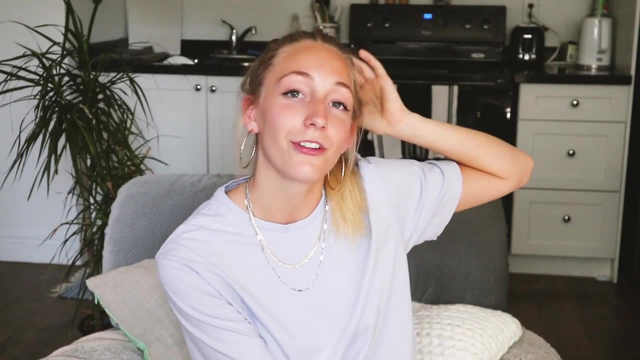 outline. It covers basic graph theory, which- don't let that fool you, because when I read this I was like: oh my god, graphs- fun. You know what you get to do with graphs, You get to color them in and you get to draw things And, being the artistic person that I am, I was so excited. 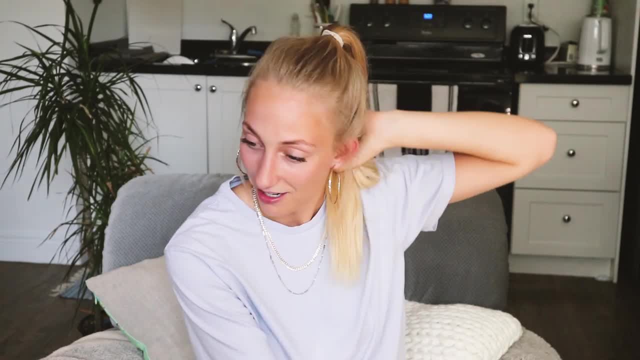 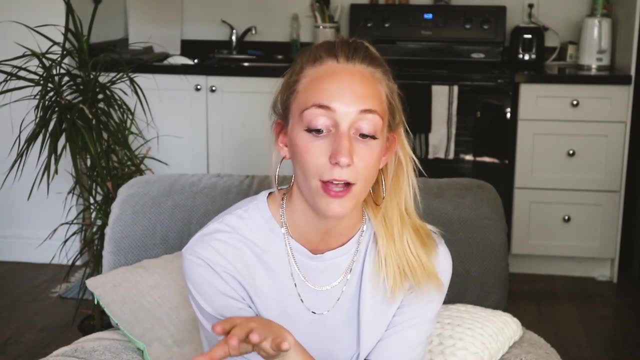 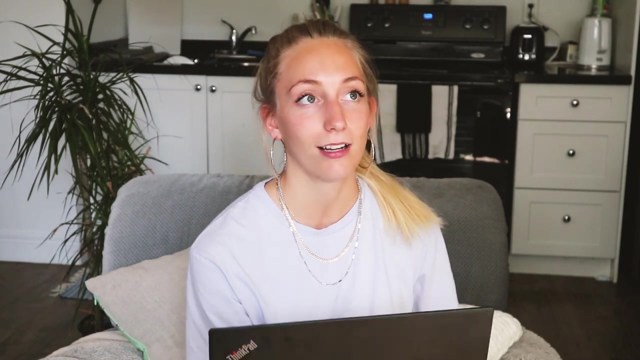 to be able to do some graphs, But it's a little more complicated than that. We worked with Euler circuits and Hamilton cycles in graphs- planar graphs. We did graph coloring- also fun. That part was pretty fun. I like that, But it's not like coloring graphs so that they're pretty. 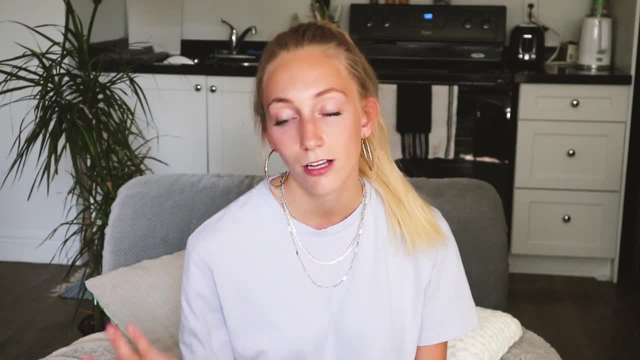 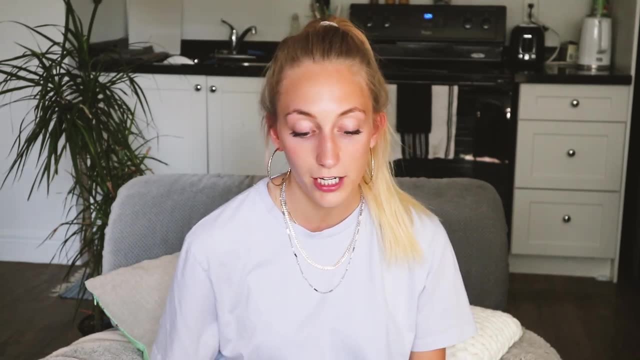 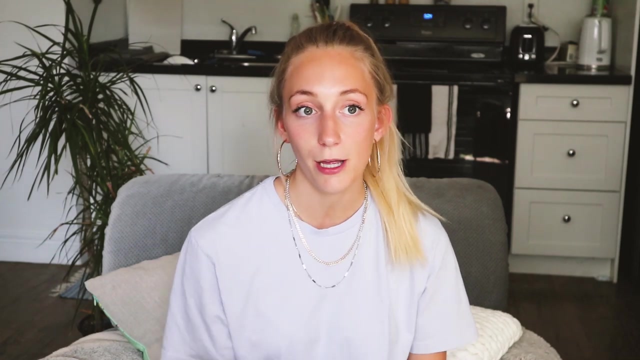 using colors to define what types of graphs. they are Not quite as interesting, but that's okay. We worked with trees, relations, partial orders, an introduction to counting, recurrence relations. we used the inclusion exclusion principle. So the prereq proofs, mathematical proofs. 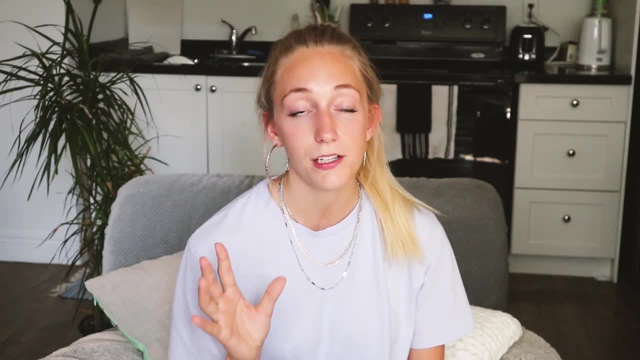 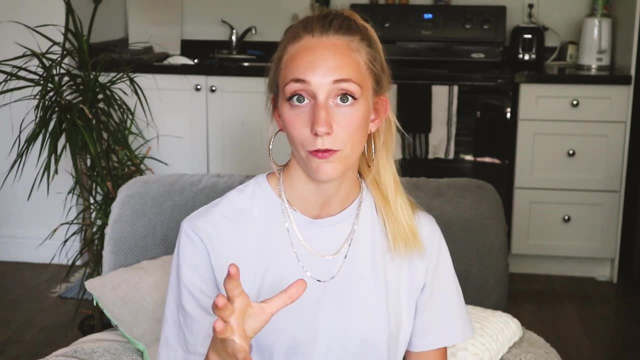 was actually a prerequisite for this course, Though this course is not nearly as wordy as mathematical proofs was. it was just a prereq because we had to prove a lot of properties, So we had to prove a lot of properties and we had to prove a lot of properties. 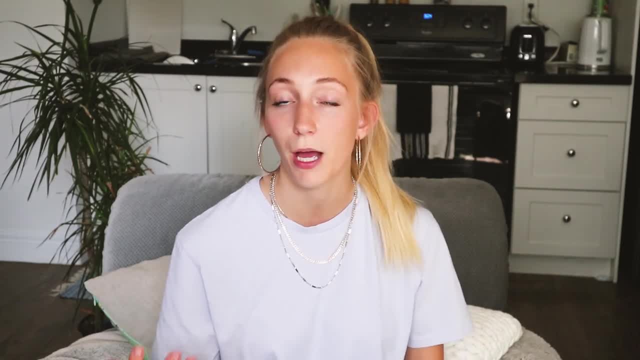 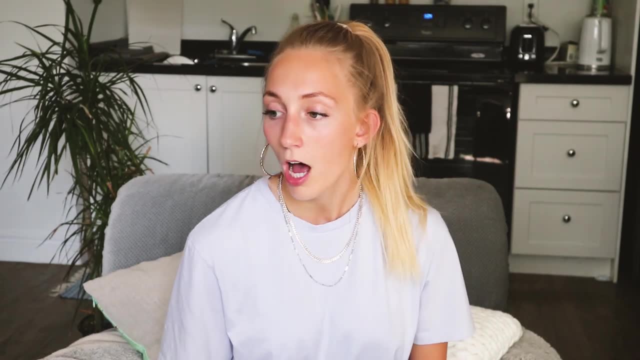 about the graphs that we were working with, So it was very helpful to have mathematical proofs. It was set up as most of the math courses normally are: We just had like a bunch of quizzes and then our midterm and our final. I don't think it was overly difficult, I don't. I think I did. 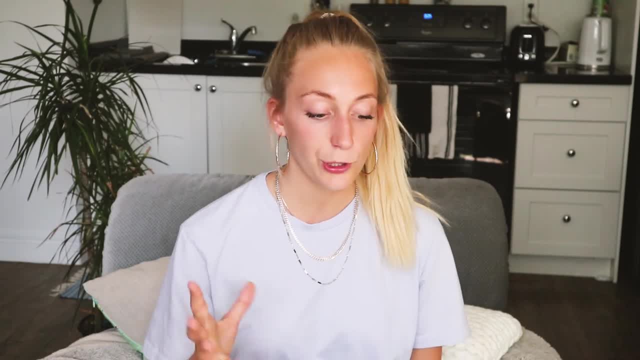 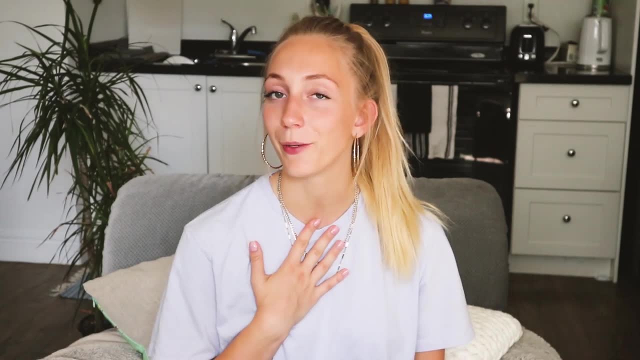 pretty well in that one as well Did not find it too bad, Even when you think about when you have like your introduction to Euler circuits and Hamilton cycles and that kind of thing. it's almost fun because they're based off of you know like little puzzles and stuff Like the. I think 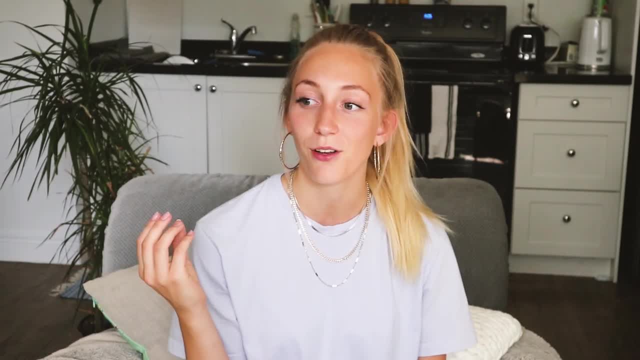 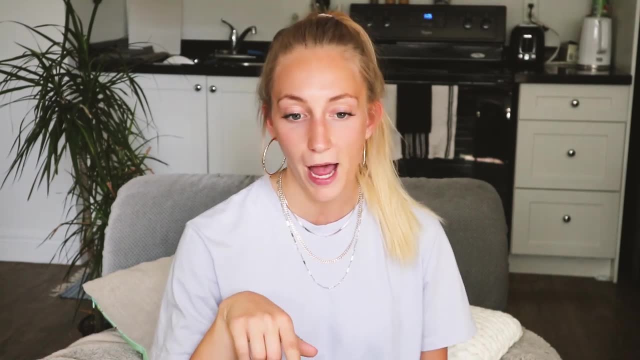 Euler, I don't even remember now. I think it's the Euler circuit that was based off that little puzzle where you have, like, villages around a river and bridges that cross the river in certain places and you have to find a path that goes to every single house or to every single village without 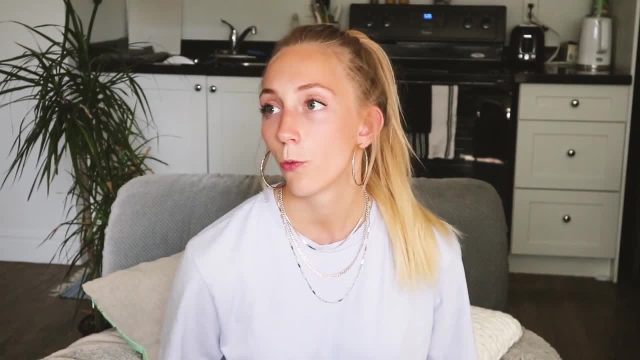 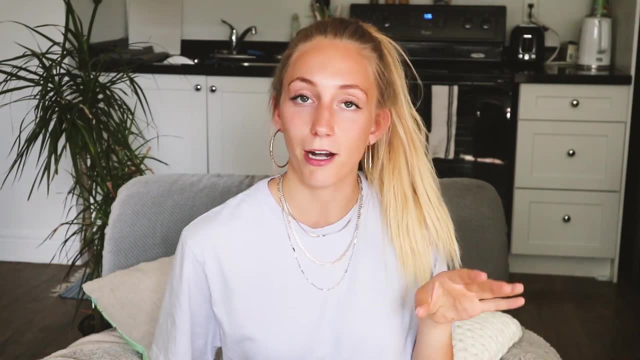 like crossing over itself. It's like fun little stuff like that, which those? that's the kind of math that I do enjoy, because it's like fun little problem solving things, But those like little mathematical games and stuff And I think it's really cool to learn about And I think it's 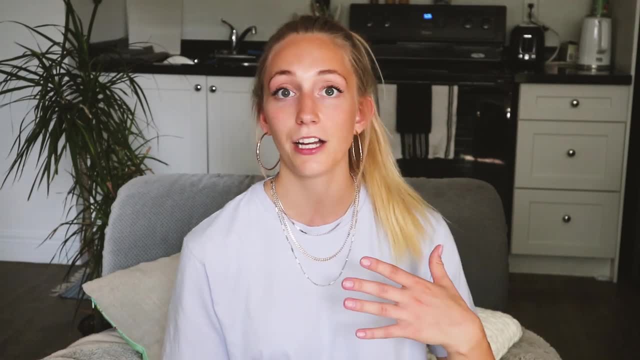 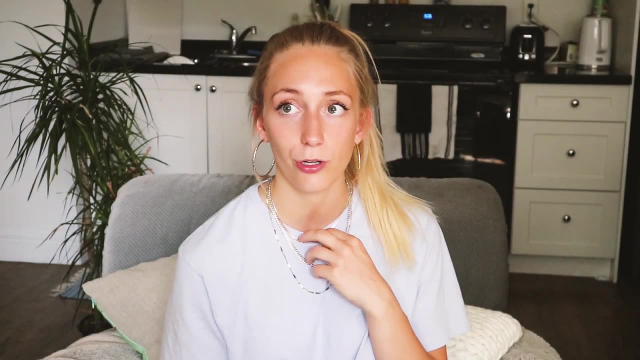 really cool to learn about And it's. they're topics that can be applied to algorithms that you may be working with in computer science And also- I actually genuinely do think- in other areas of life. if you have to do any sort of calculations or tracking or that kind of thing, it genuinely 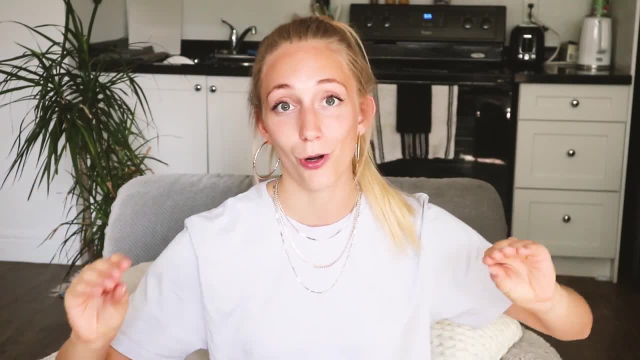 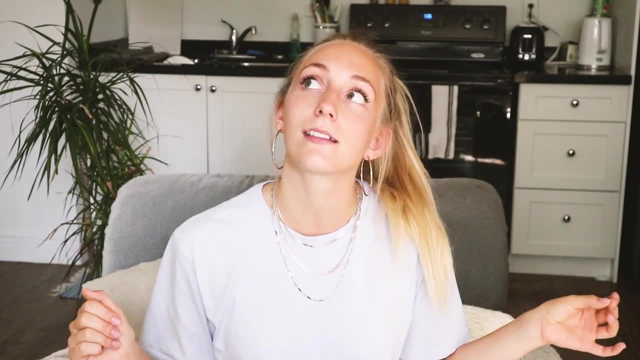 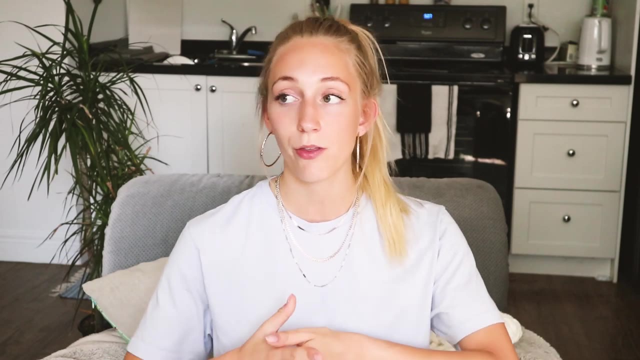 is really, really helpful and not too difficult of a course whatsoever. So we did have a textbook. It was called discrete mathematics and its applications, And we used these seven, seven, seventh edition Just to like kind of bring it back to the actual name of the course, which is discrete mathematics. 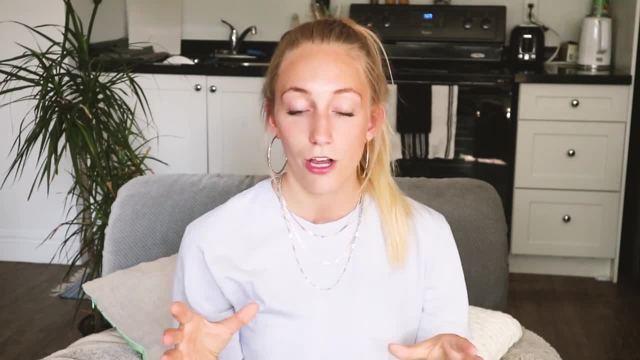 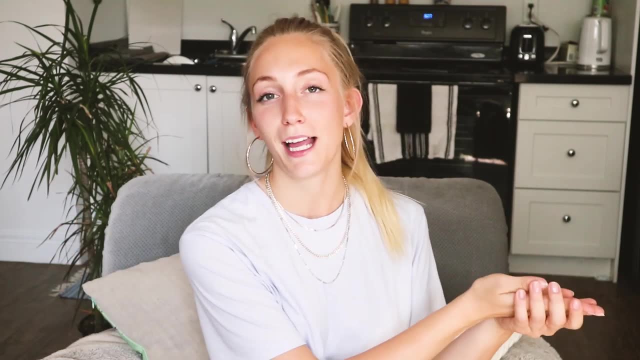 They're generally pretty good, easy numbers to work with. So, like if you think about discrete data versus continuous data- at least when I think about it- there are a lot less. there's a lot less jumble of stuff that you have to work with If everything is discrete because it's all set. 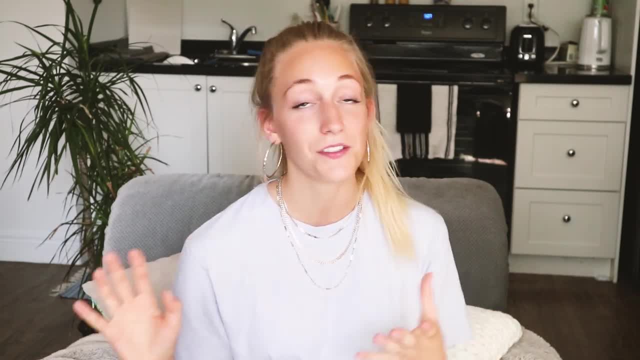 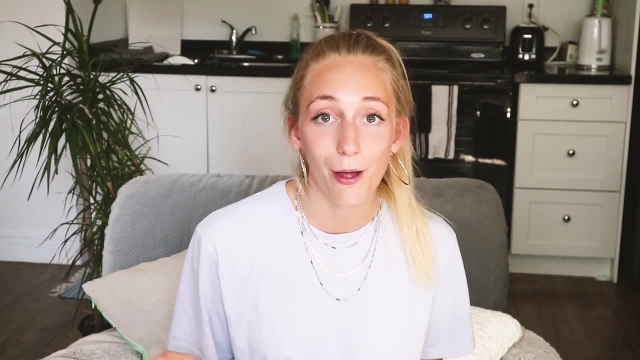 static numbers, they're all particular, separate values, Whereas continuous data, like on a graph, you know these three data points and then every single infinite number in between. So I also really liked working with discrete math. just because of that They were very simple numbers. 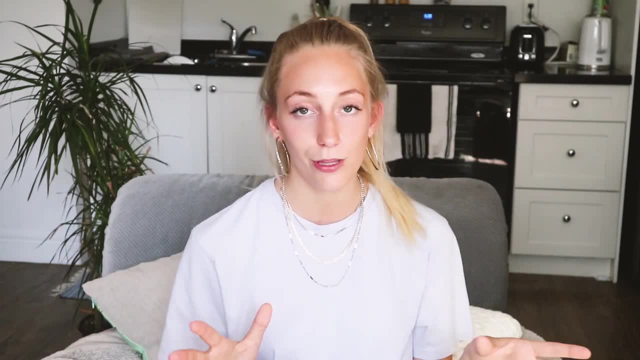 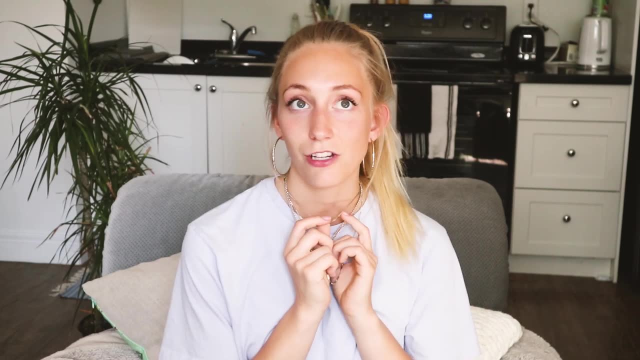 and it was more um patterns and puzzles and little algorithms that you could work with. So I enjoyed that one. I mean, like it's funny now that I'm saying I enjoyed it, because when I was in the class I don't think I was enjoying it at all. but like you get through it, you know. 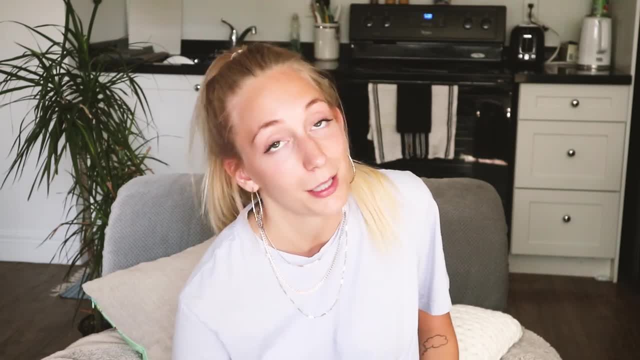 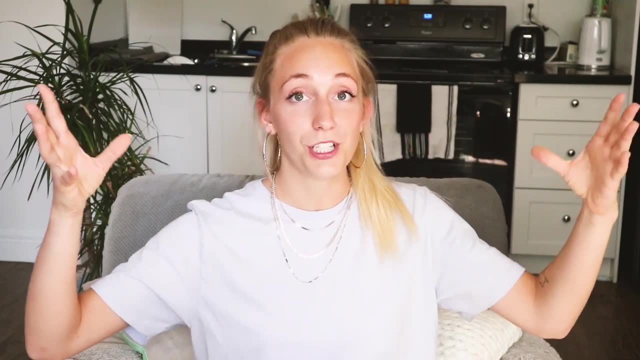 all of these classes, like you get through and then you're like: shoot, maybe that's kind of helpful, Except for calculus. Yeah, Thank you guys for so much for sticking with me through all of these course breakdowns. I know it's been a lot and um, given that I just filmed like seven of them. 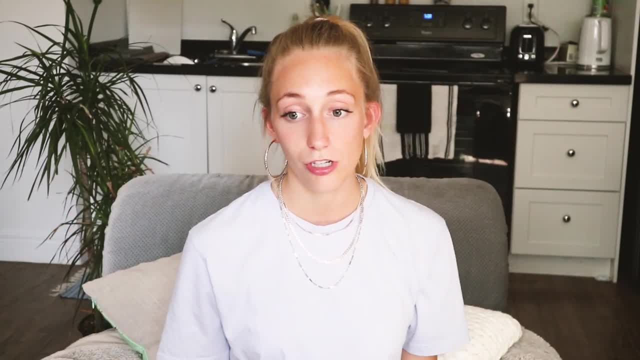 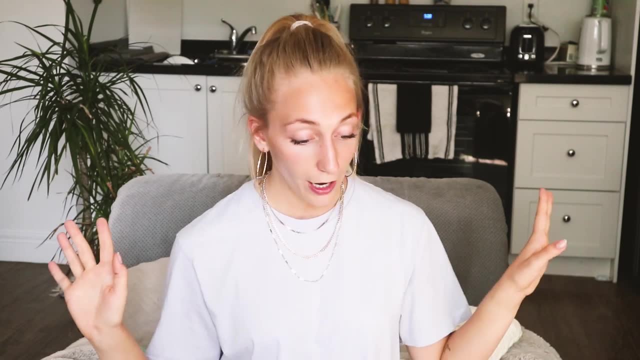 I think, um, I know that there's going to be a whole bunch that will be all up at the same time. I know that's a little bit of a mess, but I do want to get them up for you guys, So hopefully that's okay. It is not okay. It sucks to suck. They're there. Thank you guys. 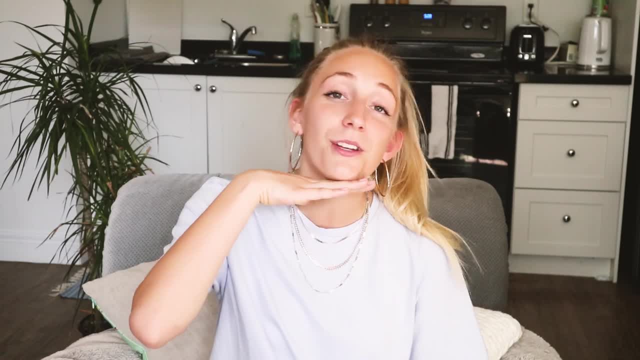 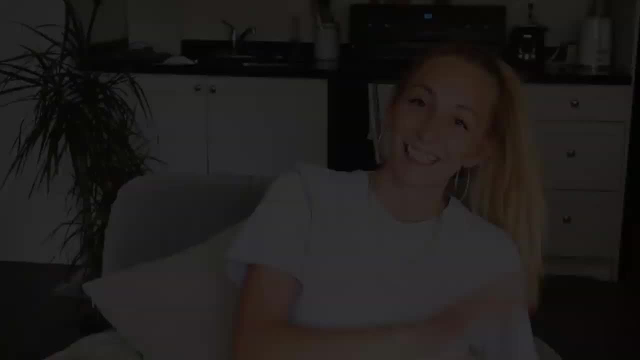 So, so, so, so much for watching. Don't forget to smile, and I will see you all in my next video, which is not going to be a course breakdown. Ooh, I'm tired. Bye.